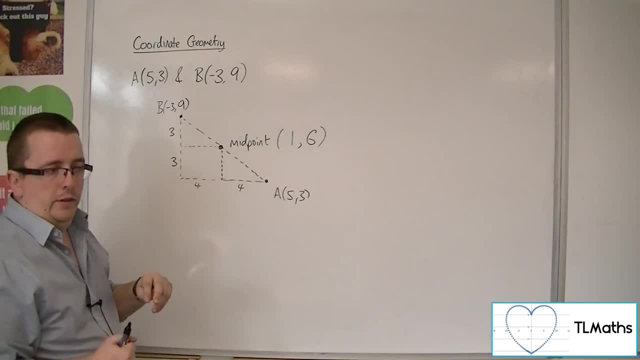 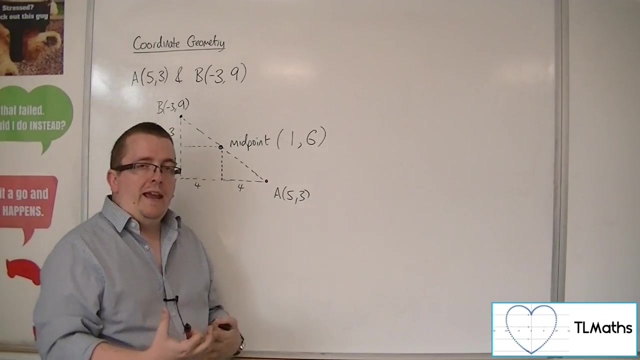 So the midpoint is definitely 1, 6.. Now it would be nice if there was a faster way for me to find this midpoint, rather than having to draw a triangle and find it this way. So, as I said, this midpoint is like the average of the two coordinates. 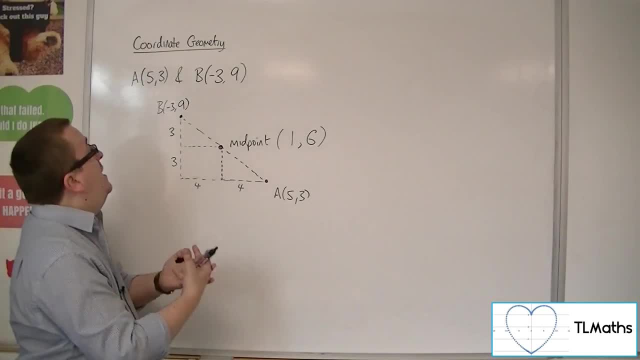 It's the mean of the two coordinates. So if we add the x-coordinates together and divide by 2, I will have the average of the x-coordinates. And if I add the y-coordinates together and divide by 2, I'll have the average of the y-coordinates. 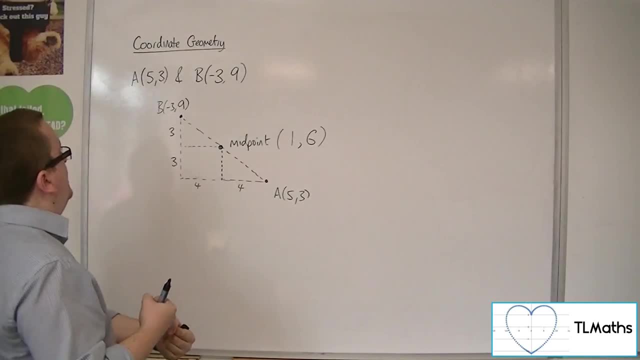 So I'll have the average of the x and the y and that will give me my midpoint. So you can think about finding the midpoint as a coordinate. So you can think about finding the midpoint as a coordinate by adding the x-coordinates together. 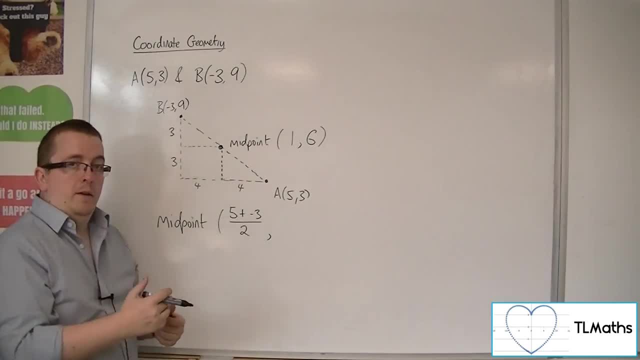 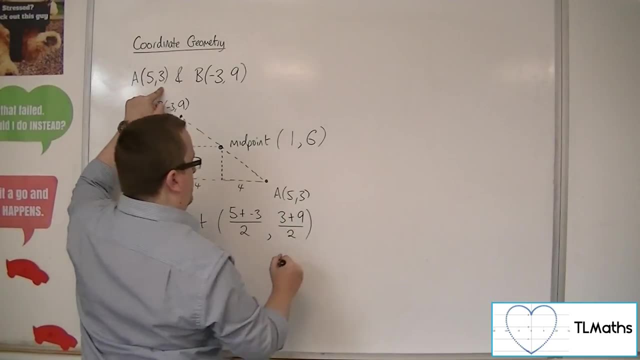 So 5 plus minus 3.. And then dividing by 2. So you're dividing by how many there are, And then I've got 3 plus 9.. divided by 2. And then I've got 3 plus 9.. 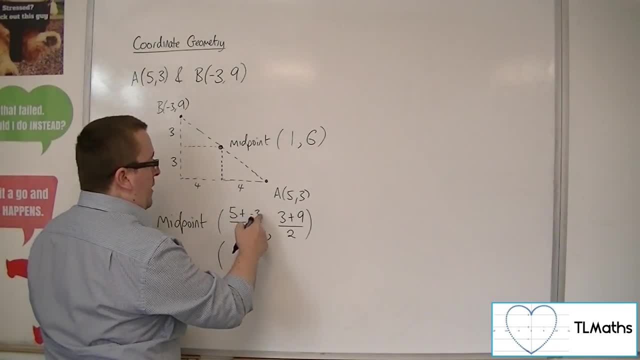 divided by 2. For the y-coordinates, And so we would have 5 plus minus 3.. So 5, take away 3, which is 2, divided by 2, is 1.. So 5, take away 3,, which is 2, divided by 2 is 1.. 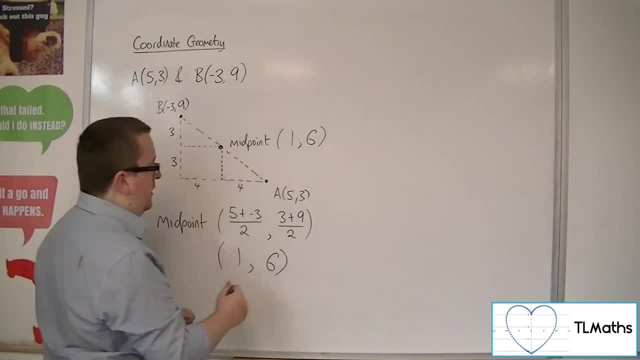 So 5, take away 3,, which is 2, divided by 2 is 1.. So 5, take away 3,, which is 2, divided by 2 is 2.. So, if I remember that, that is the way to find the midpoint. 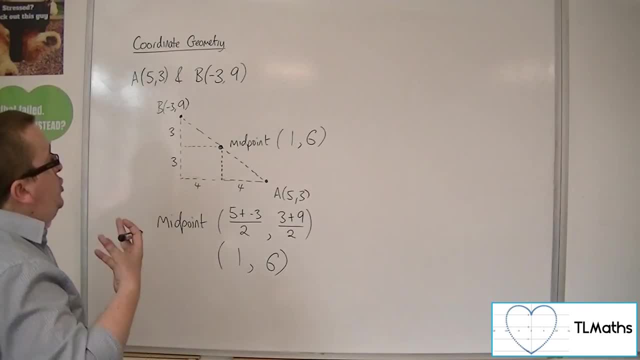 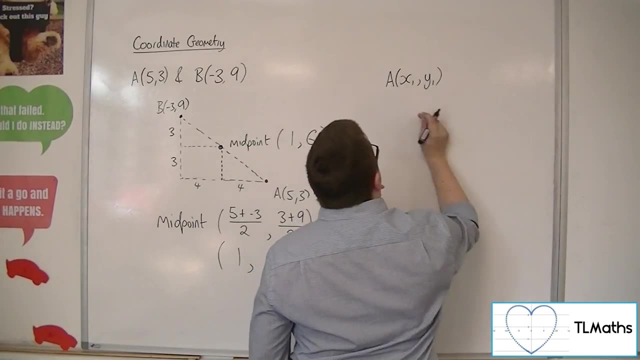 I can find it relatively easily, So that in general I can find it relatively easily. So let's say we've got the 2's co-ordinates, so let's say we've got A. so let's say we've got A. 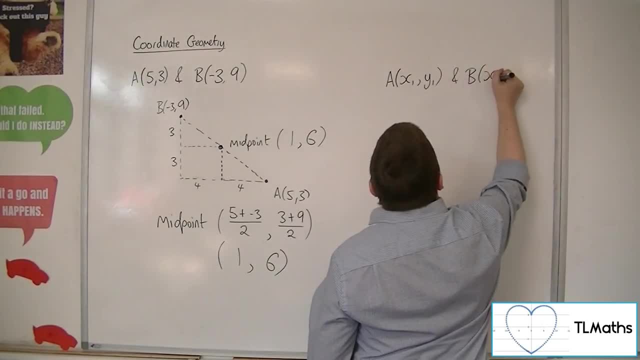 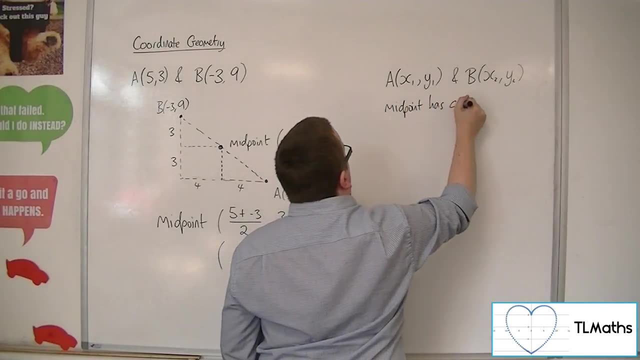 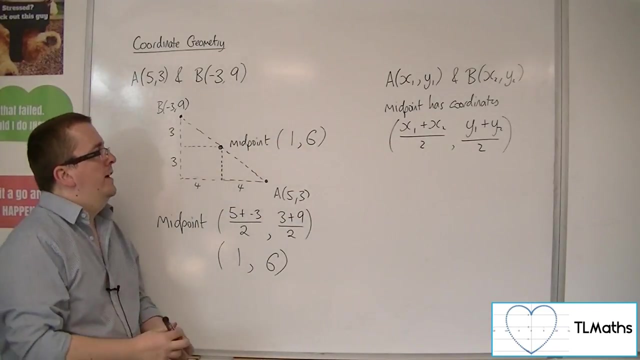 is at the general co-ordinates and B, which is at x2, y2. then midpoint coordinates x1 plus x2 over 2 as the x-coordinate and y1 plus y2 over 2 as the y-coordinate, And that's how we can find the midpoint between any two coordinates.